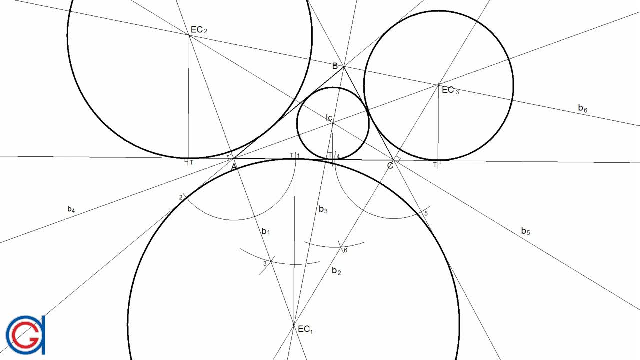 called the x-center. The in-center is located at the intersection of the three external angular bisectors. The three x-centers are located at the intersection of the internal bisector and external bisector of the two other angles, Because the internal bisector of an angle is perpendicular. 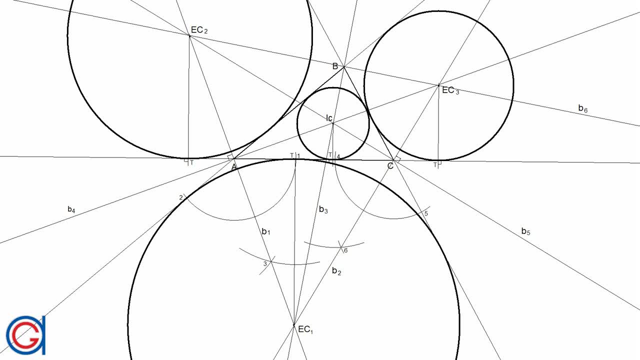 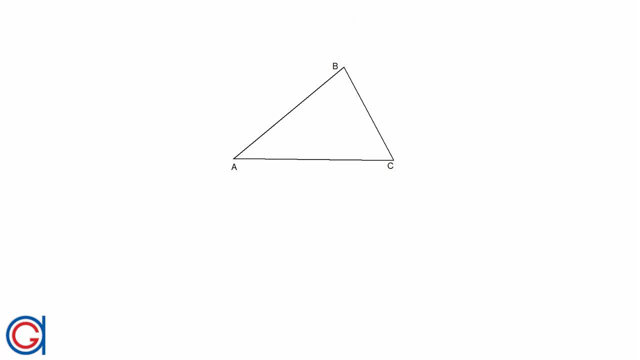 to its external bisector. it follows that the in-center together with the three x-centers form an orthocentric system. So, to start, we are going to elongate the three sides of the given triangle with construction lines using a ruler, as can be seen here. 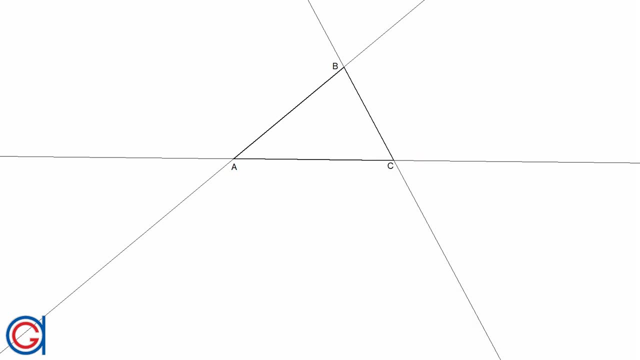 So, to continue, we are going to work out the external angular bisector of the vertices A and C. So, setting the compass on point A and with a random radius, we draw an arc, obtaining points 1 and 2, as can be seen here. 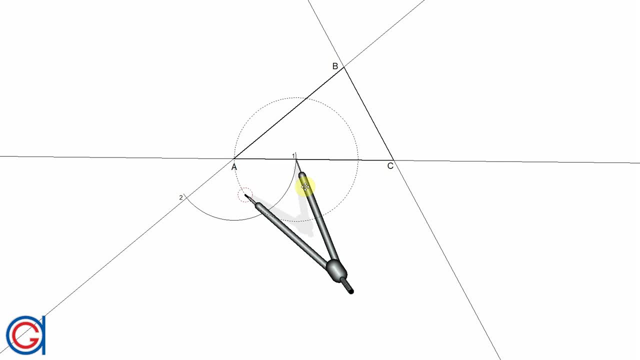 And now, setting your compass to a slightly larger radius and setting it on point 1, we scribe an arc as shown. Now, setting your compass to a slightly larger radius and setting it on point 1, we scribe an arc as shown. 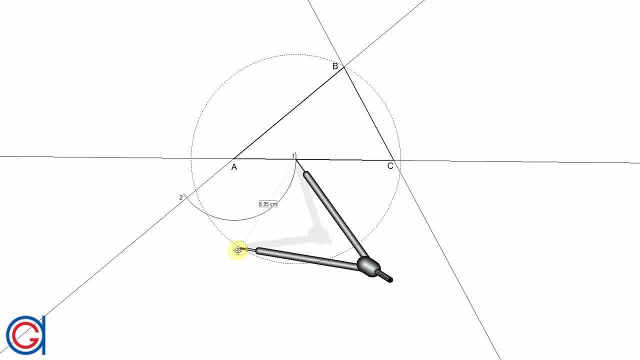 And now, with the same radius and setting on point 2, we scribe another arc, cutting our previously drawn arc at a new point, which we will call point 3.. So now, with the ruler, we join vertex A to point 3 and elongate it as shown here. 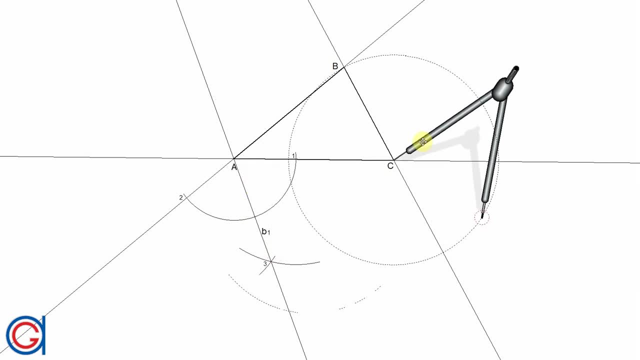 And we will name this bisector B1.. Now we are going to repeat the same process With vertex C. so, setting your compass on the point C and with a random radius, we draw an arc, obtaining points 4 and 5, as can be seen here. 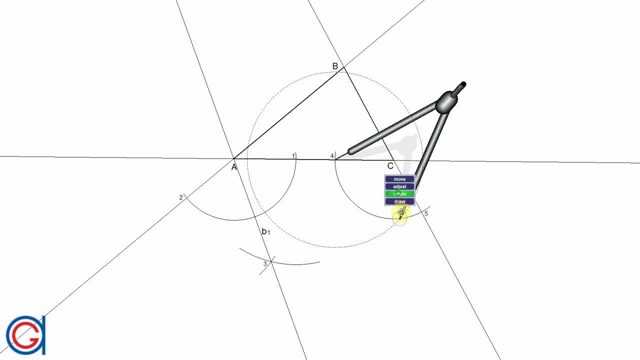 And now, setting your compass to a slightly larger radius and setting it on point 4, we scribe an arc. And now, with the same radius and setting it on point 5, we scribe another arc, cutting our previously drawn arc at a new point, which we will call point 6.. 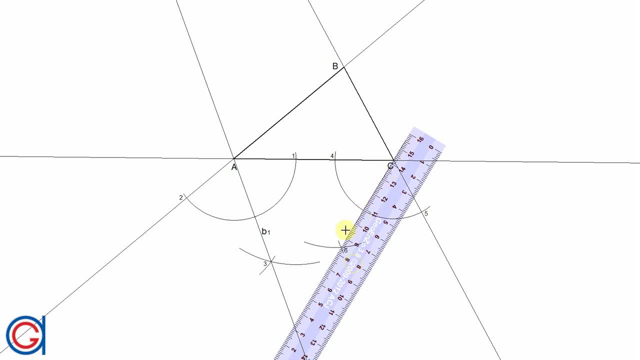 And now with the ruler, we join vertex C to point 6 and elongate it on both sides as shown, And we will name this bisector B2.. And where these two bisectors intersect is going to be the first x-center of the x-circle. 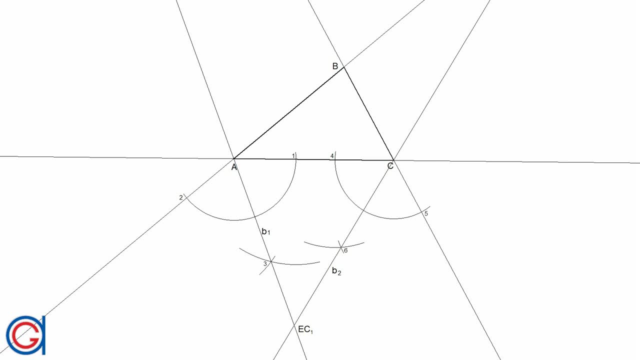 to the side AC and we will call it x-center 1, or EC1.. So to obtain the internal angular bisector of vertex B, you only have to join points B and EC1, and elongate it on both ends, and we will call this line B3, or bisector 3.. 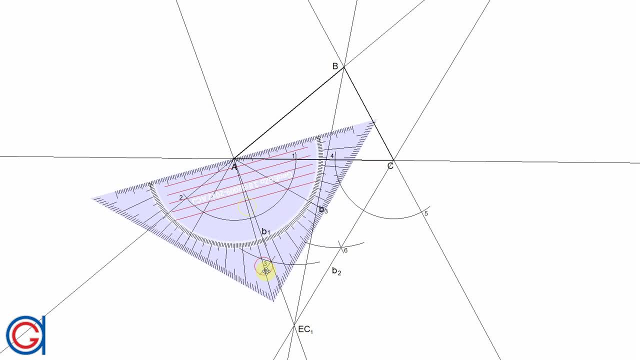 So to obtain the internal angular bisector of vertex A, you have to draw a perpendicular line to B2.. We will call this line B1, passing through points A and elongate it on both sides, and we will call this angular bisector B4.. 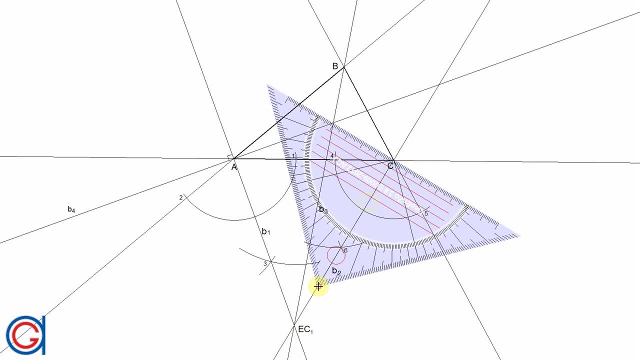 So now we are going to repeat this process with vertex C, drawing a perpendicular line to B2, passing through point C, and elongate it on both sides, and we will call this internal angular bisector B5, as can be seen here: 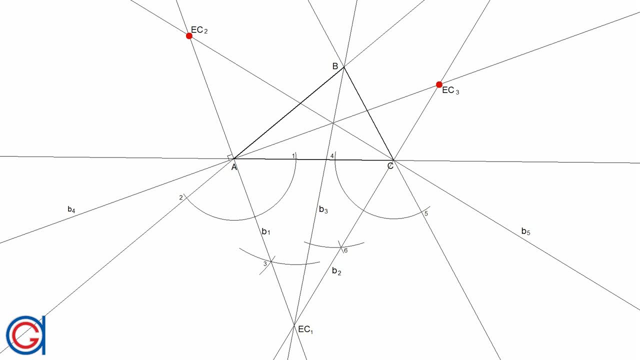 With these angular bisectors, we obtain two remaining x-centers, highlighted here in red, and the in-center highlighted in blue. So now, joining EC2 and EC3,, we are going to get the last angular bisector, which we will call B6, and elongate it on both sides again. 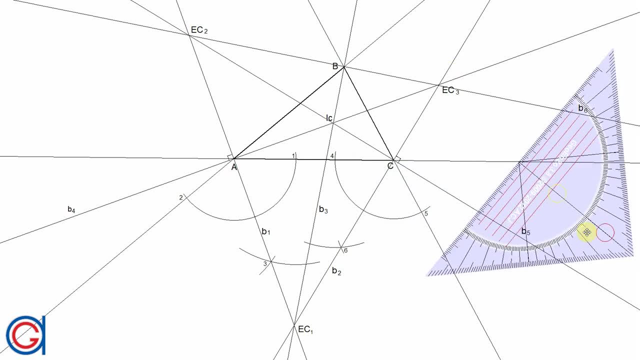 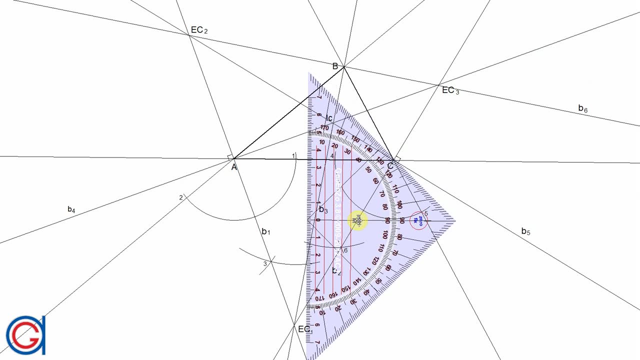 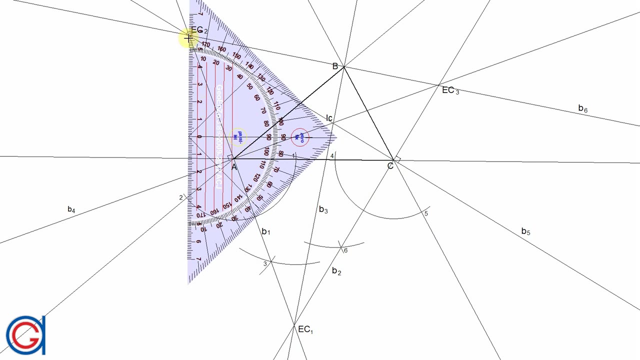 So the next step is to draw perpendicular lines to the AC axis, passing through each of the three x-centers and the in-center, in order to obtain four radiuses of the circles that we want to draw. Where this line cuts the AC axis will also be the four tangent points and also the length. 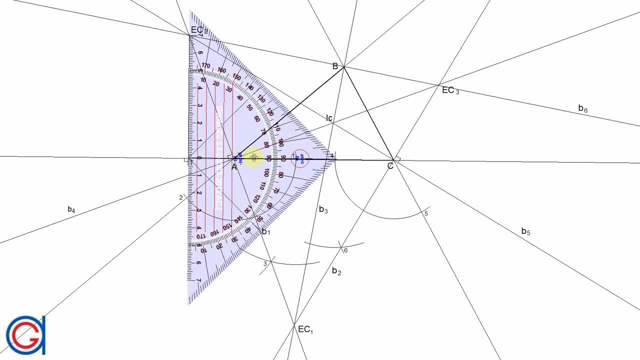 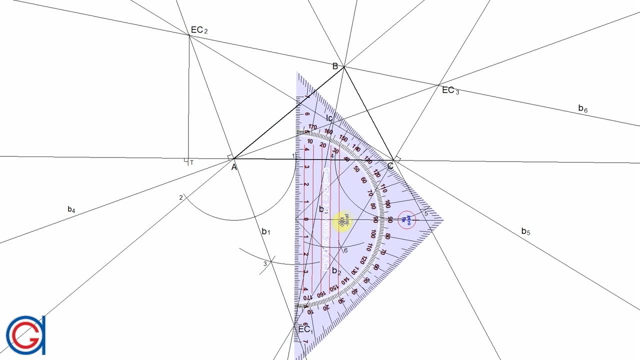 of the radiuses of each circle that we want to draw. So with the ruler we draw a vertical line from EC2 to the AC axis, obtaining our first tangent point and the length of the first circle and again joining EC1 to the AC axis. 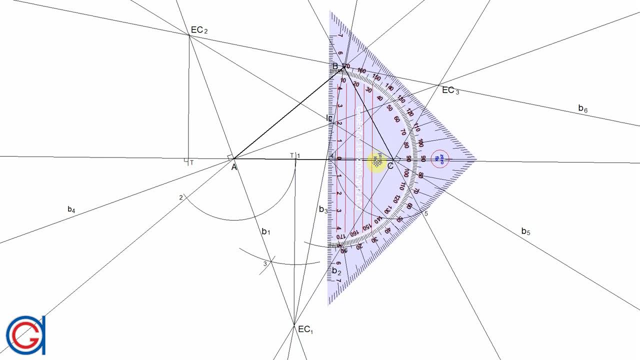 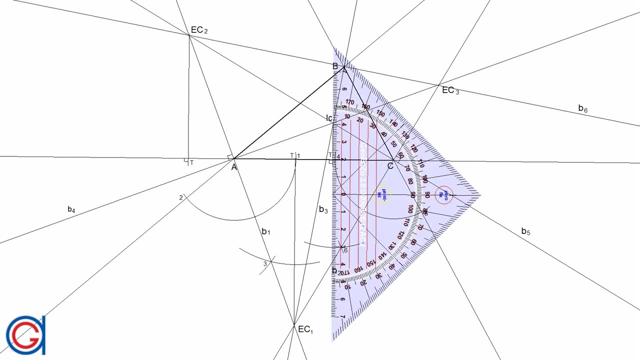 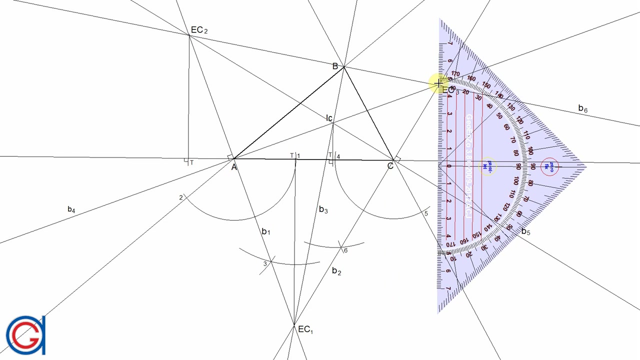 we obtain our second radius and second tangent point. Now, joining the in-center to the AC axis with a perpendicular line, we obtain another tangent and another radius of the in-center circle. Finally, joining the x-centers- constraint 3, to the AC axis with a perpendicular line 이. 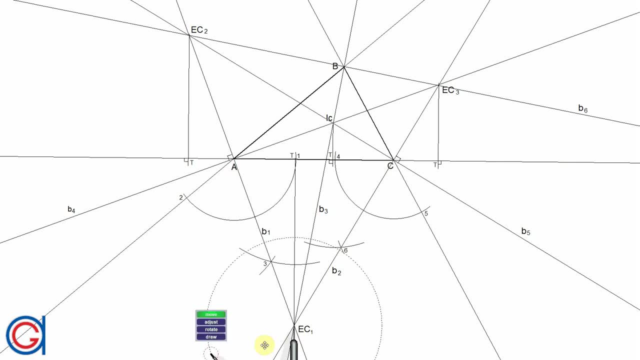 ller Jeju 7結・F3 Remain. thank you a lot for reminding me this step of making circuit tangent point and the fourth radius. so now setting our compass on ec1 and with the radius ec1 to the tangent point on the ac axis, we draw a circle in a thicker line, as can be seen here, and to get our 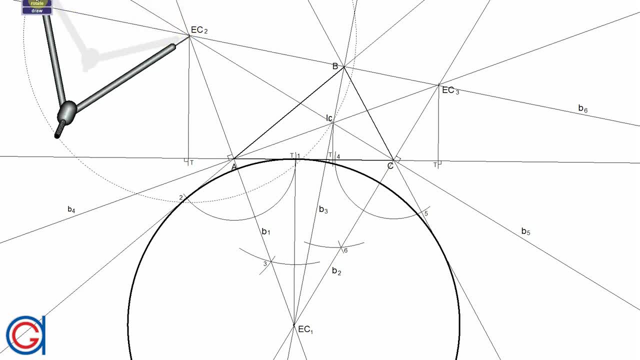 second circle, setting the compass on ec2 and with the radius ec2 to the tangent point. we are playing before we draw our second circle in a thicker line, as can be seen here and now. setting the compass on the third x center, ec3, and with radius ec3 to the 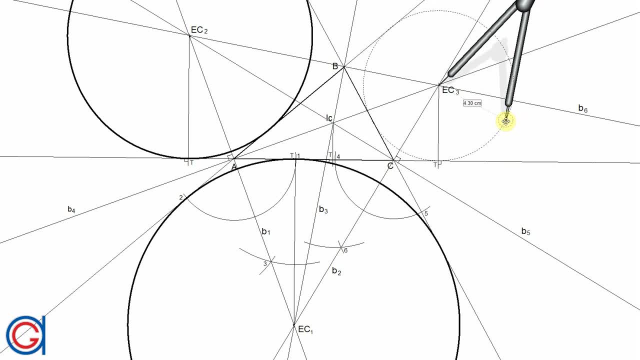 fourth tangent point, we will draw in a thicker line our third x circle, as shown here. and finally, setting our compass on the in center point ic, and with the radius ic to the third tangent point, we draw our final in circle in a thicker line, as shown here. 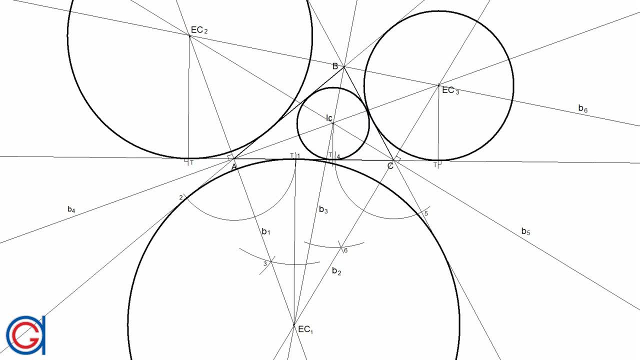 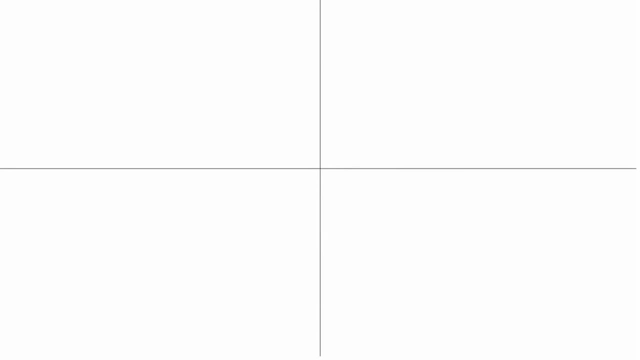 so here we have the in circle and the three x-circles of a given triangle ABC. I hope this video has helped you. Please press like or subscribe to our YouTube channel Until the next video. thank you, Thank you.